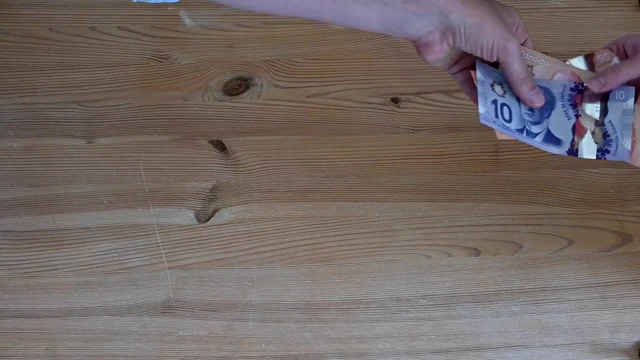 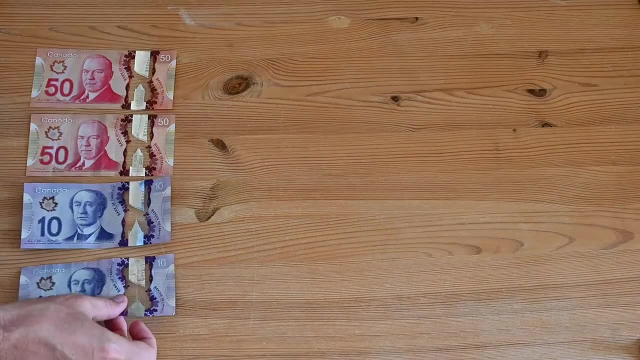 year. you owe me the original hundred dollars and ten dollars in interest. you owe me a hundred and ten. If the loan is for two years, you'd owe me the original hundred, the ten percent interest for the first year and another ten percent interest for the second year, a total of one hundred and twenty. 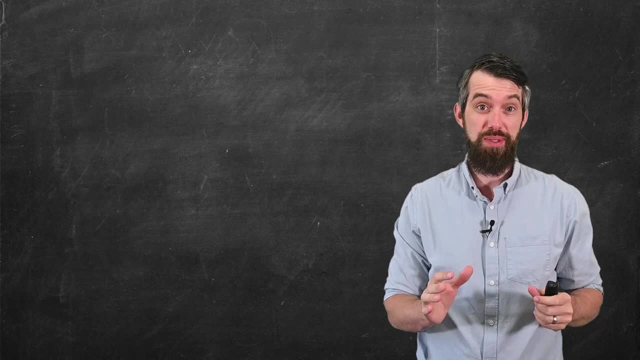 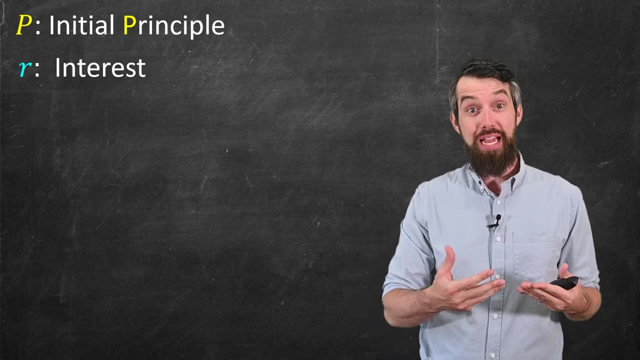 So let's try to come up with a formula for this. Let me establish a few terms. I'm going to let P denote the initial principle. For example, a hundred dollars would be the amount that would be loaned out, and then R stands for the interest rate. so for example, ten percent interest in some. 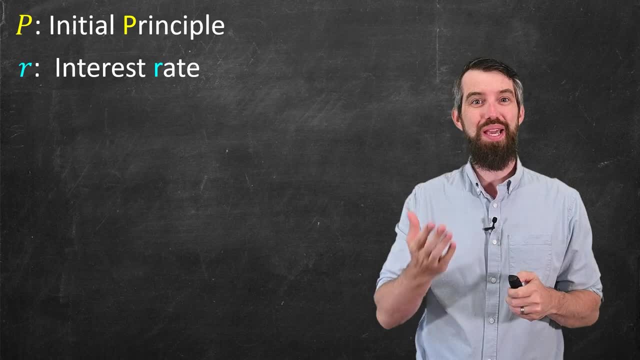 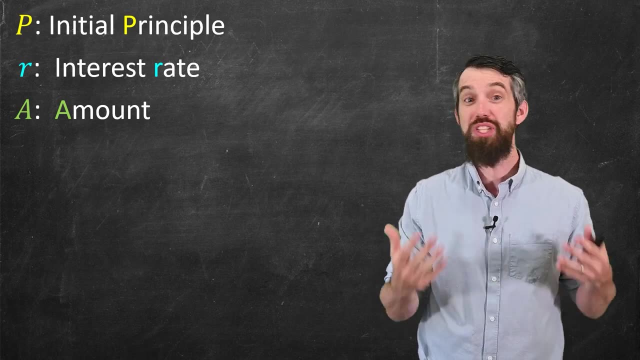 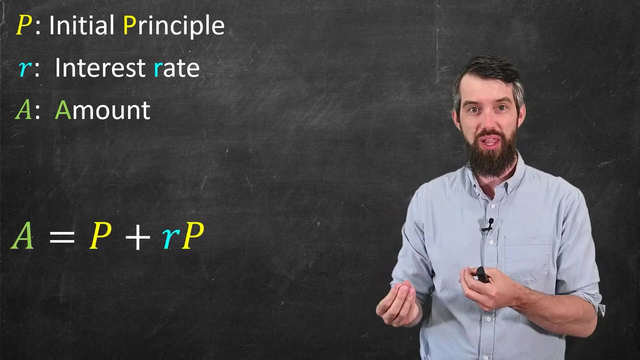 period like a year, and then what I want to know is the amount A that I'm going to get back. So if I loan out my money, what's the amount that I'm going to receive? So what's a good formula for this? Well, I'm going to say that the amount A should be equal to the principle plus R times the principle. 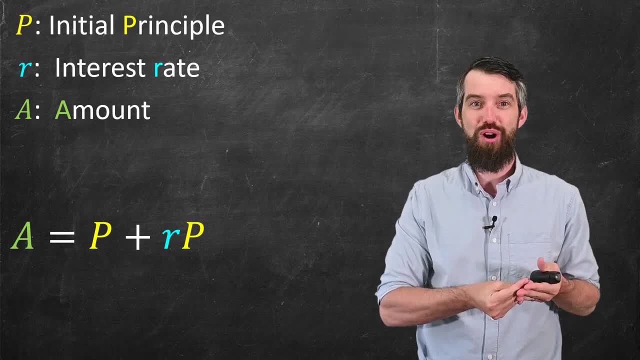 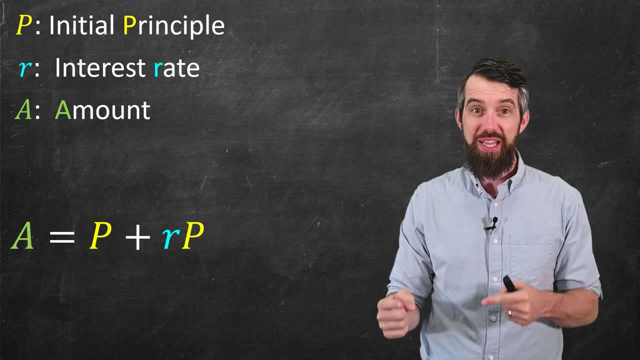 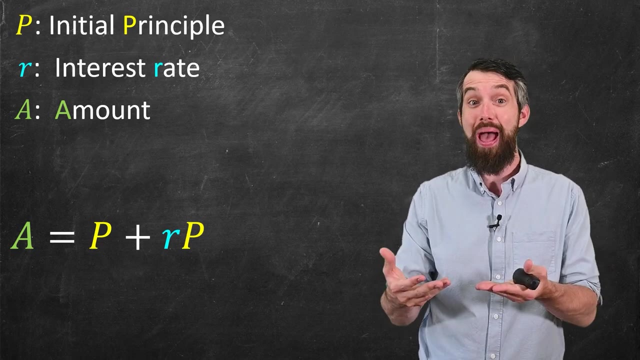 What's the idea here? Well, the first P stands for: if I loan out a hundred dollars, I better get that back. I better get back my initial principle. and then the RP stands for the interest I get. So, for example, if my interest rate is ten percent, then I would get ten percent of the principle back. as 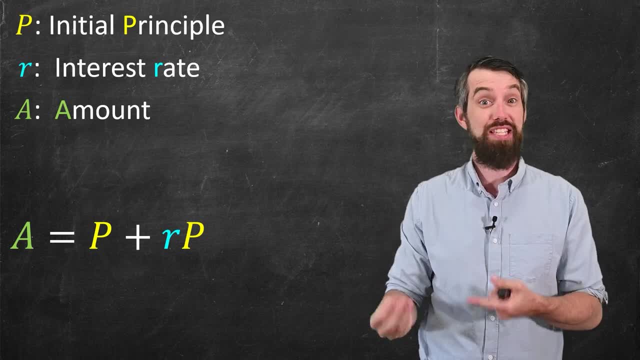 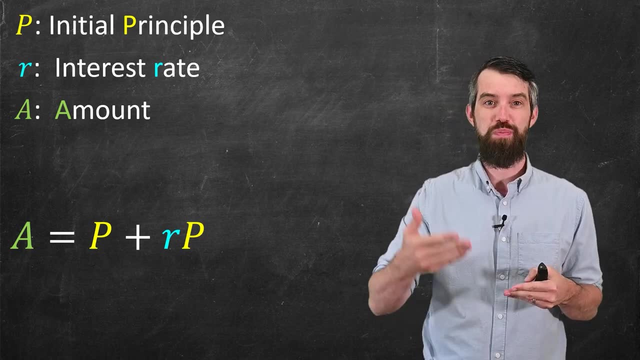 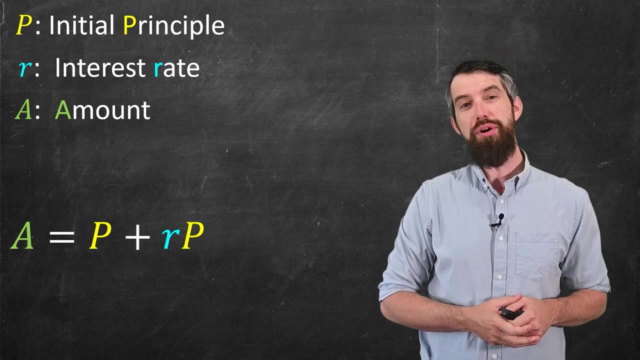 interest in addition to the initial principle. This gives me the final answer that I would get back P plus RP. But now I want to imagine that I loan the money out for multiple periods. So, for example, if it's ten percent per year, maybe I loan it out for two years, and if I loan it out for 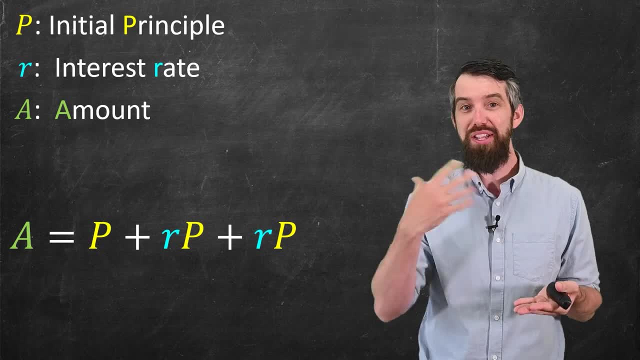 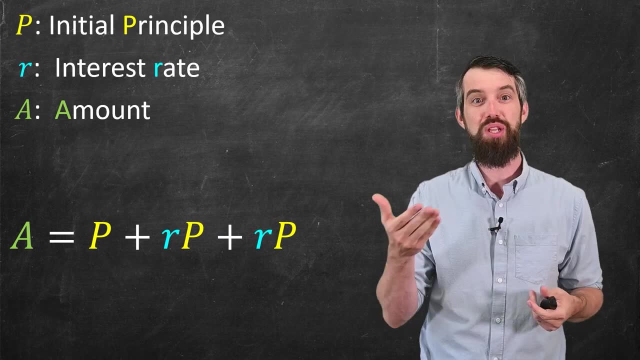 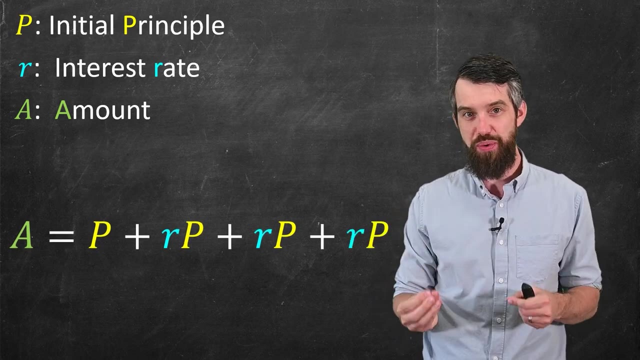 two years I get my initial principle P back. I get one year of interest growth RP back and then a second year of interest growth, another RP, and so I get P plus RP plus RP. If I lend it out for three periods I'd have another RP and in general I can keep on doing this and the magic of simple. 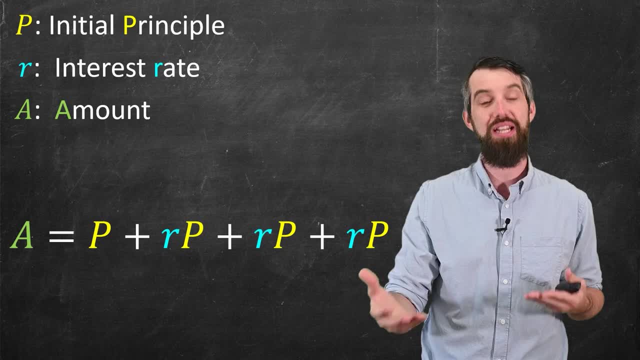 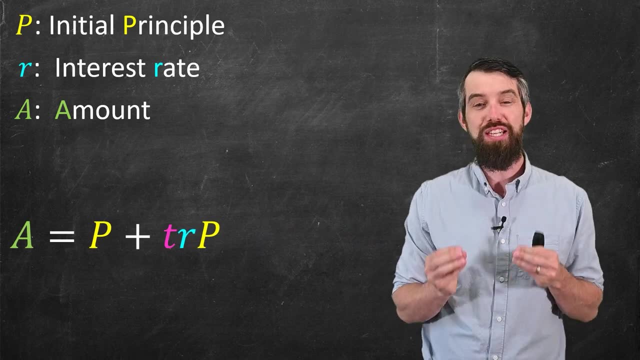 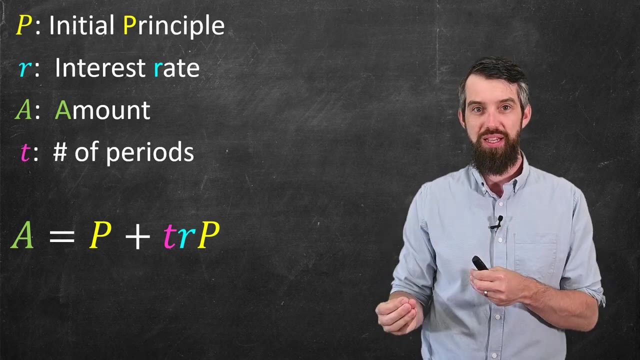 interest here is that every time you go forward another period into the future, you just have the same interest payment, RP- over and over again. And that lets us simplify our formula. Our formula can just be P plus T times RP, where T is the number of periods. So, for example, if your period is a, 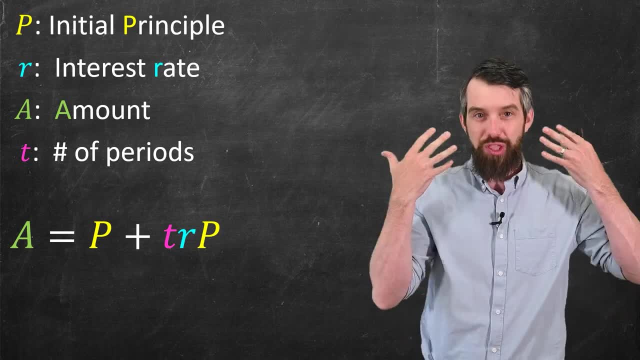 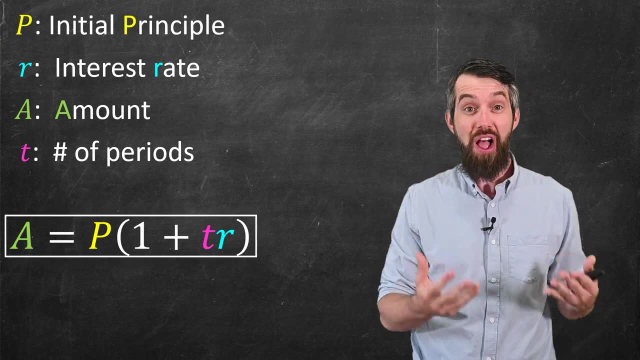 year and you loan it out for three years. then you get your principal plus three times RP. I notice that there's actually a P in both factors here, so I can just factor it out and I get my final formula for simple interest. Okay, so that's the formula, but let's try to build a bit of an. 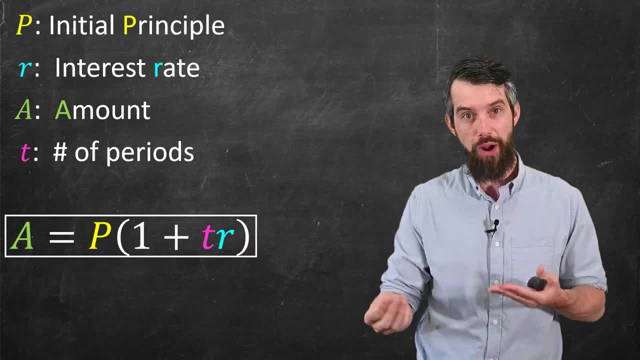 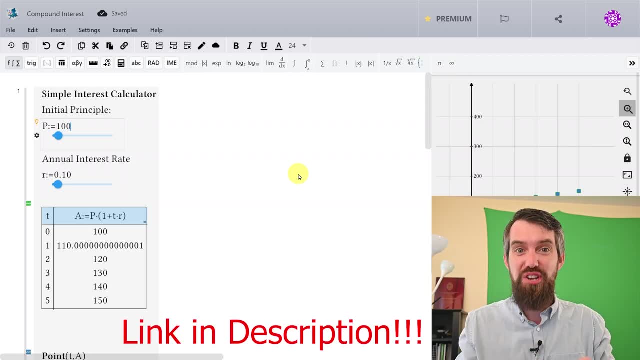 intuition for how quickly this simple interest is going to grow. I've built a simple interest calculator in MapleLearn- and MapleLearn is actually the sponsor for today's video. So down in the description you can check out this exact workbook where I have my simple interest calculator, my 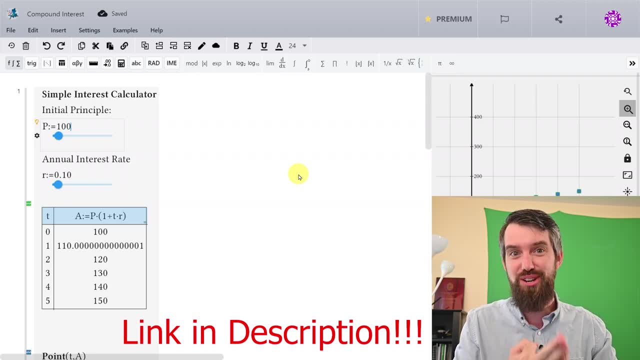 compound interest calculator and my continuously compounded interest calculator. MapleLearn is a web app that allows you to make these interactive math workbooks where it does all of the computations for you. They're really cool, so check them out. Now, what I've done here is I've made a 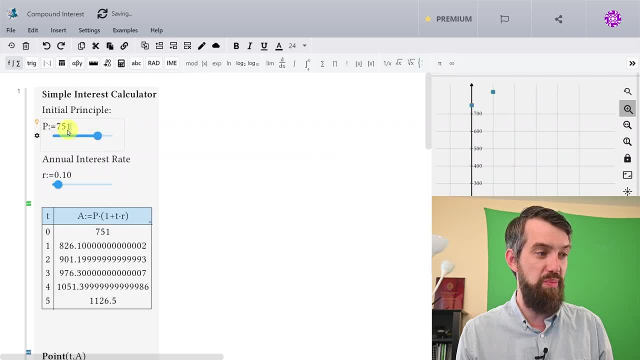 couple different sliders. So, first of all, you can set your initial principal to be whatever you like. You can also set your initial principal to be whatever you like. You can also set your initial principal to be whatever you like. You can also set your initial principal to be whatever you like. 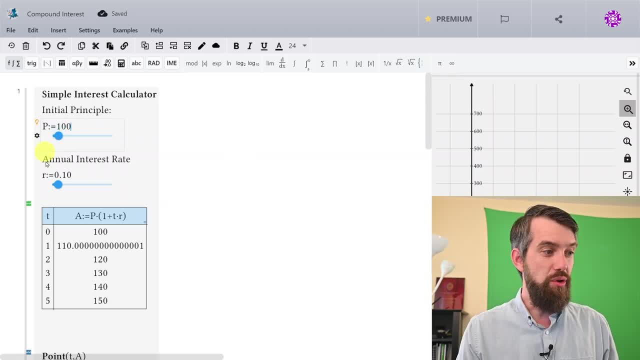 For example, the 100 that we started with sounds good. You can similarly slide your interest rate to be whatever you like. I'm going to set it back to be equal, just to 10.. And then down here you get a nice table that tells you the amount A in years: 0,, 1,, 2,, 3,, 4, and so on. What you can see is that 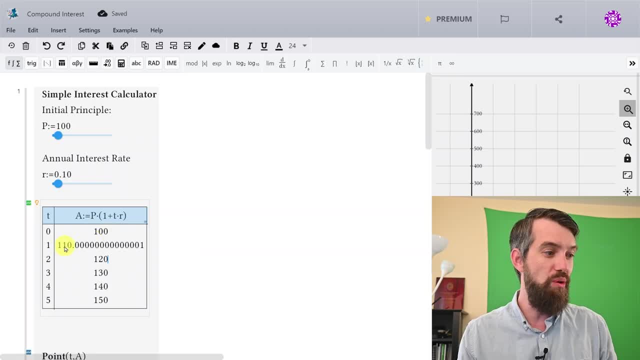 for simple interest it just goes up 10 bucks a year, 10, 1,, 10,, 1,, 20,, 1,, 30,, 1,, 40, and so on. And on the right we see a nice little plot of how it grows. as well, Pretty. 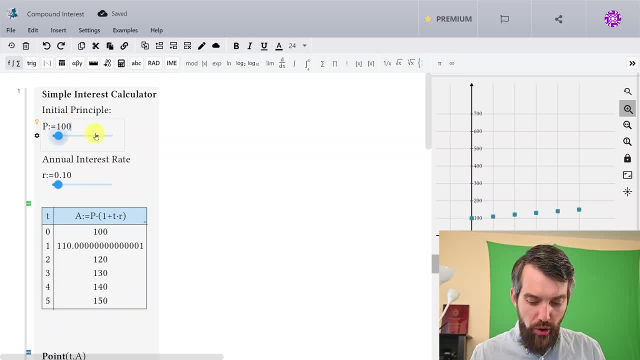 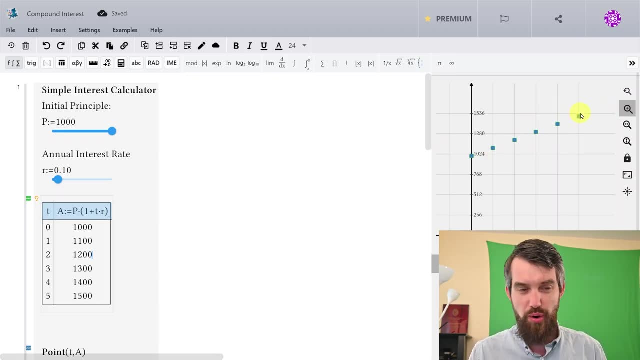 simple, And the most important part about simple interest is: it doesn't matter what you start this is. I could start this at a thousand, for example, And if I do that, well, it has the same kind of growth pattern. Just the same amount, In this case $100, not $10 now, but the same amount every. 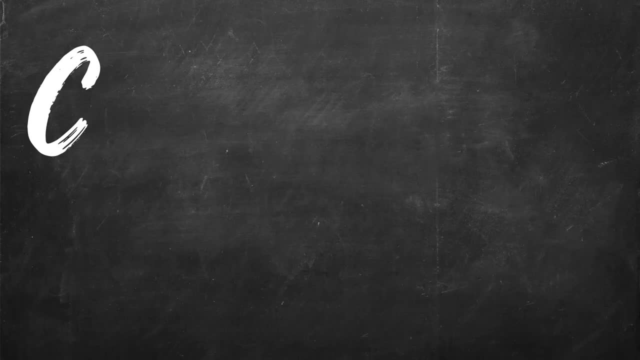 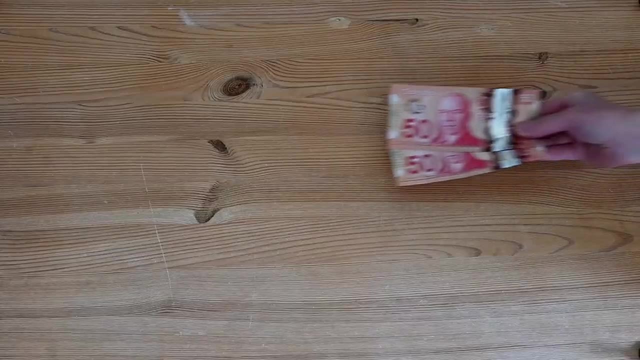 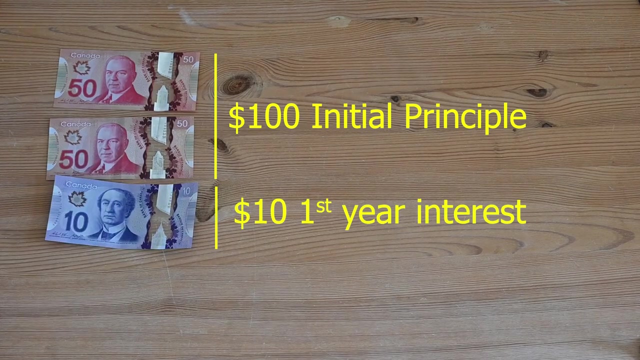 single year. It's simple interest. for a reason It's pretty simple. Now, simple interest was great, but it has a little bit of a problem. Let's imagine one period has gone by, say a year, So the $100 is now going to $110.. Simple interest would say that for the second year you'd only owe me. 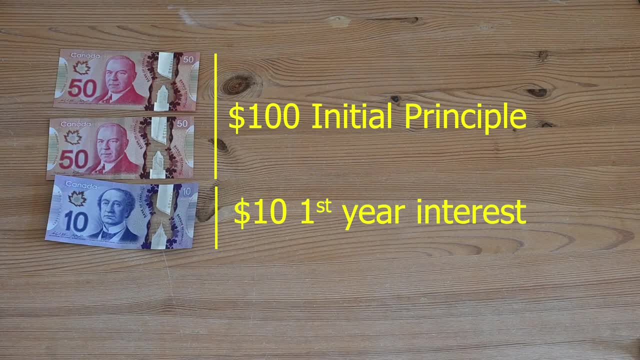 another $10. But that would only be the interest on the original $100. But you now owe me $110. So I want the full 10% on the entire $110. That is, I'm going to want $11 in my second year, So in 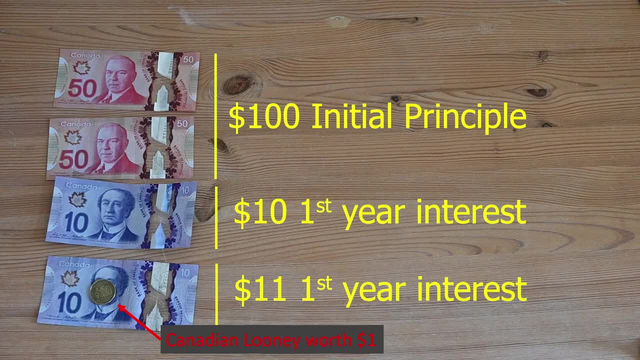 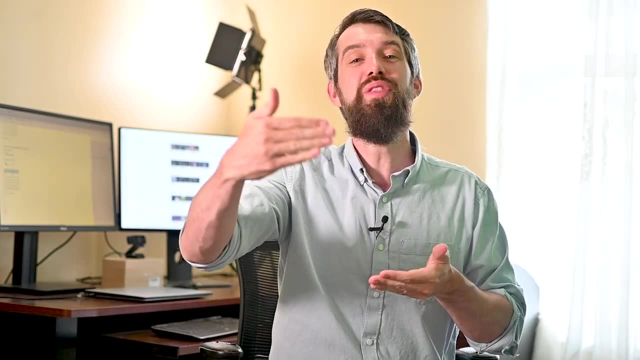 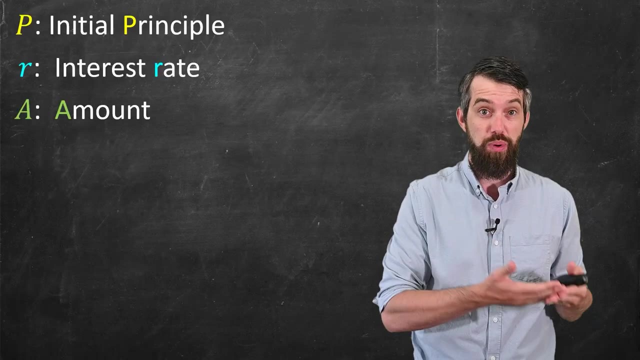 other words, it would be the initial $100, the first year's interest of $10, and the second year's interest of $110.. So I'm going to have to write down the formula for that. I again have my principle, my interest rate and the amount A at the end of my loan. Now, if I only have one period, 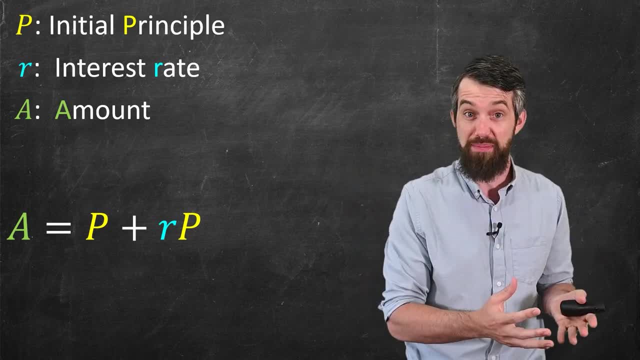 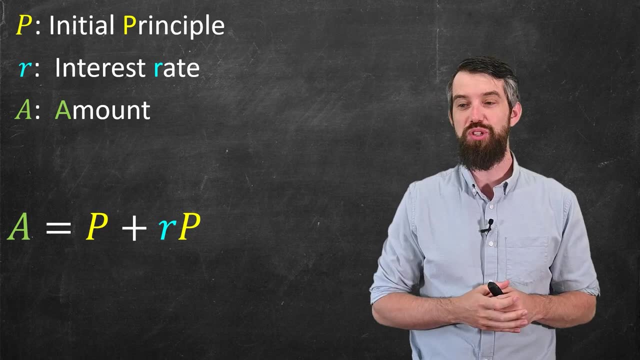 the formula is actually exactly what we saw before. The principle comes back, and then I also get an interest payment. the R times P, And I'm actually going to go and factor out the P at the beginning this time. So make this P times 1 plus R, And the way I think about this is I'm going to 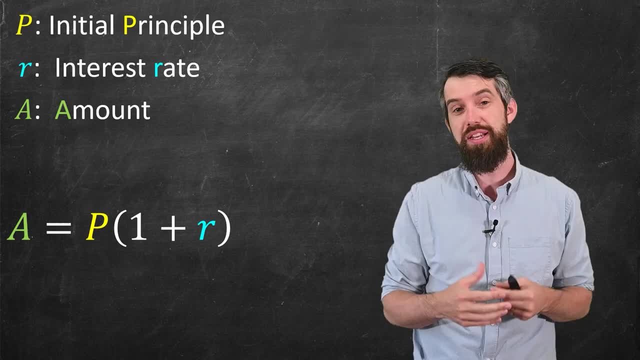 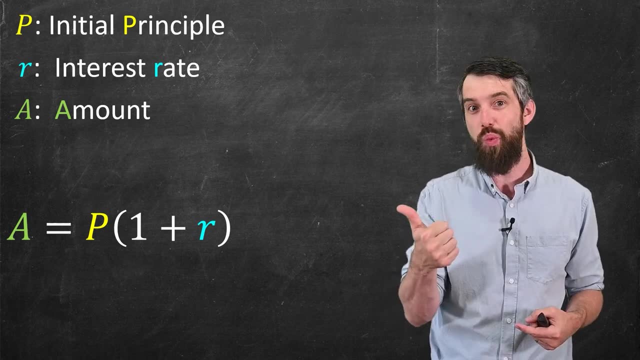 think about this is that the P represents well the amount that was lent out, And then the 1 plus R is the multiplicative factor. It says I need to get back the initial amount, that's the 1 and then also the plus R. that's going to be the interest. So if you just take the P and multiply it by 1, 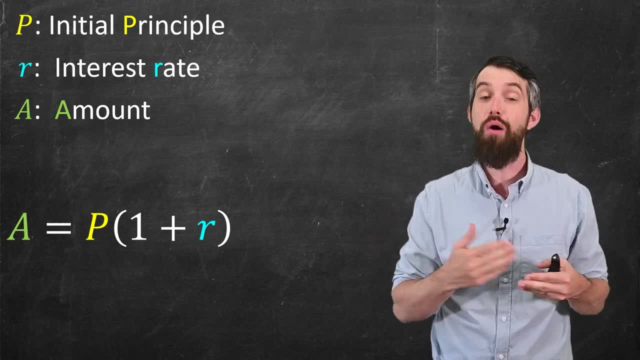 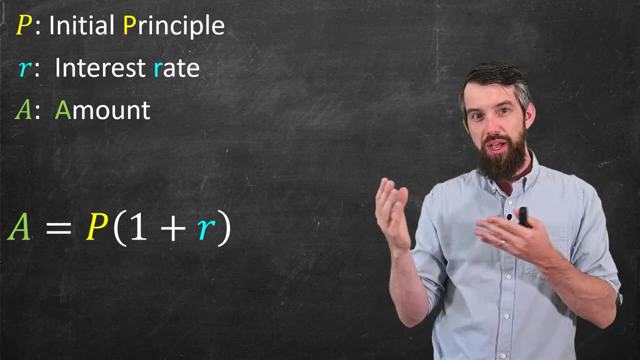 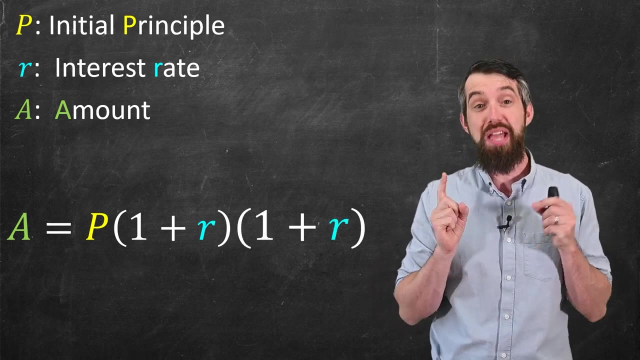 plus R, that's the new amount that's owed. Okay, now imagine I go forward not one, but two periods into the future. Well, one period in the future is this, But two periods in the future. that's how much you owe, and then I need to apply interest to it. In other words, I would multiply by another. 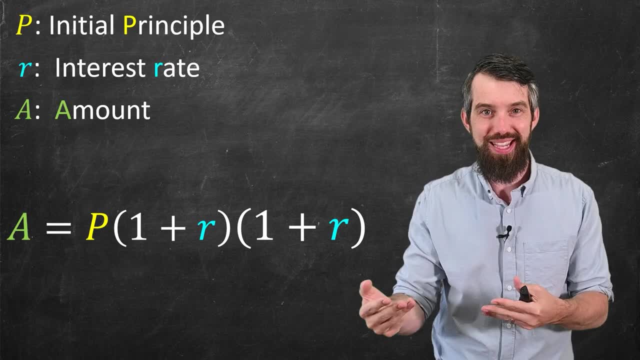 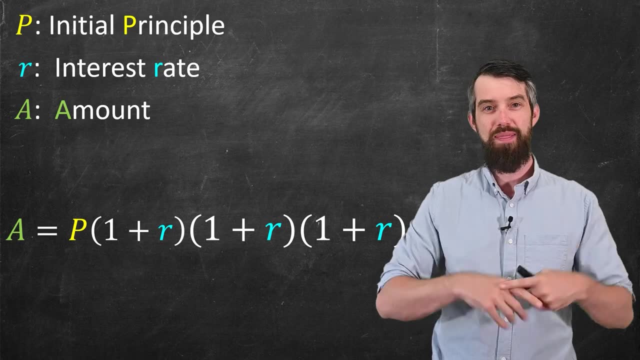 factor of 1 plus R. In fact, if I keep doing this, for example, if I go three periods, I'm going to have three factors of 1 plus R multiplied to my initial principle. The idea always is no matter what period you're on. if you go one period further into the future, you just multiply what you. 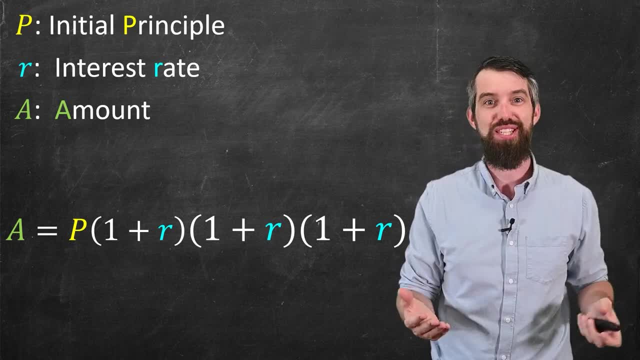 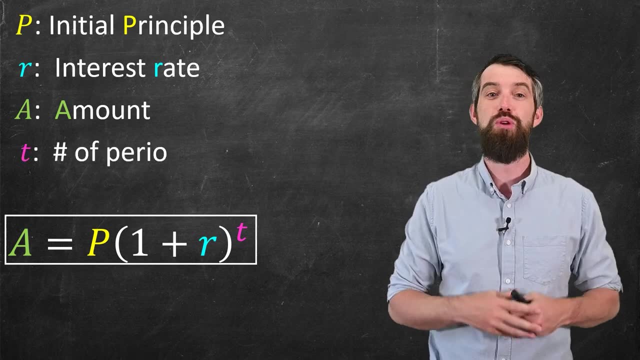 previously had by 1 plus R. And if I want to do this in generality, for a general T, I would say this is P times 1 plus R to the power of t, where t was the number of periods. Now the fact that the t is, 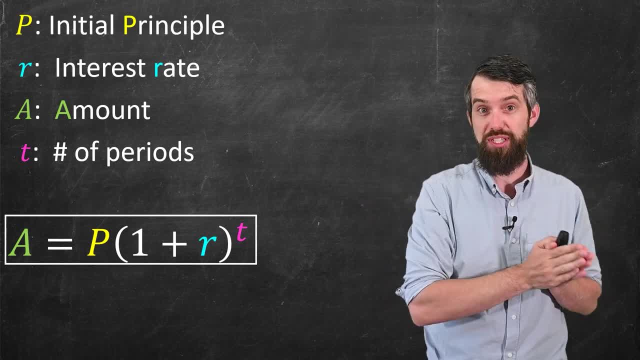 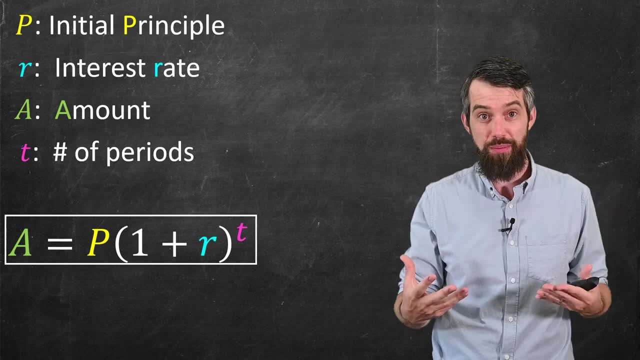 now an exponent. previously, for simple interest, it was a multiplicative factor. now the t is an exponent that is going to make compound interest grow faster. Let's see why. Alright, so back to my Maple workbook again. the link is down in. 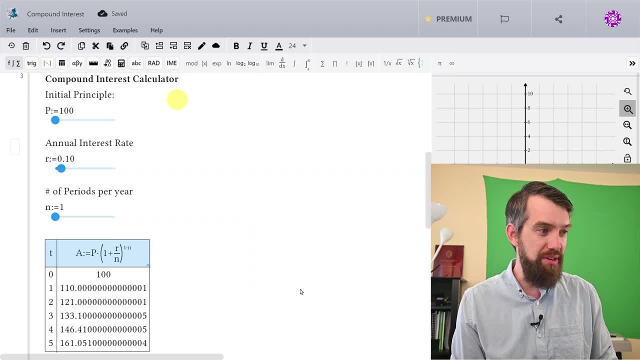 the description and I've made a new calculator for compound interest. this time I've set my principal, I sent my interest rate and then I've also had this extra factor, which is the number of periods per year, which is currently set to 1.. Don't worry about this, we're gonna elaborate this a little later on. 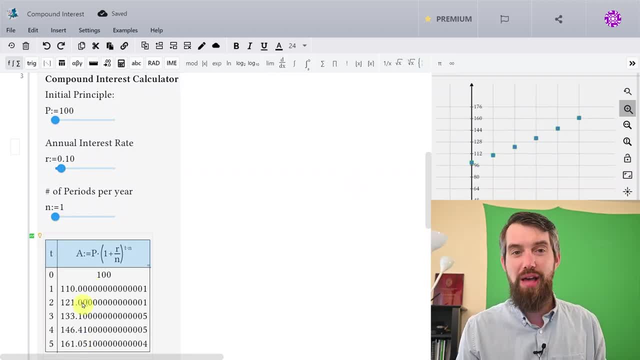 in the video, And what I again get is this nice table of values that tells me the amount a after any number of years. but what's critical here is that it's not just going up by 10 bucks every time, From 100 to 110, yes, that was 10 bucks. 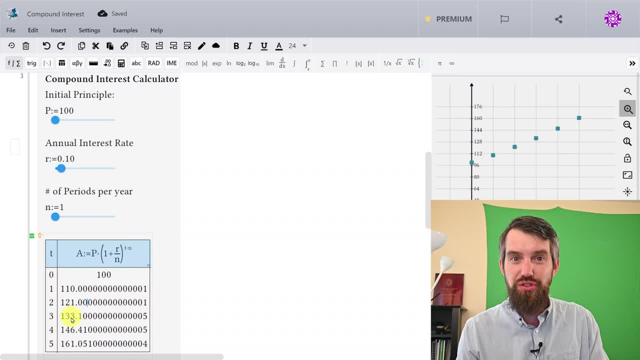 but then it goes up 11 dollars and then it goes up 12 dollars and so forth. That is the value of the interest. payment is growing every single year because there's interest on the interest And this could really matter. So, for example, 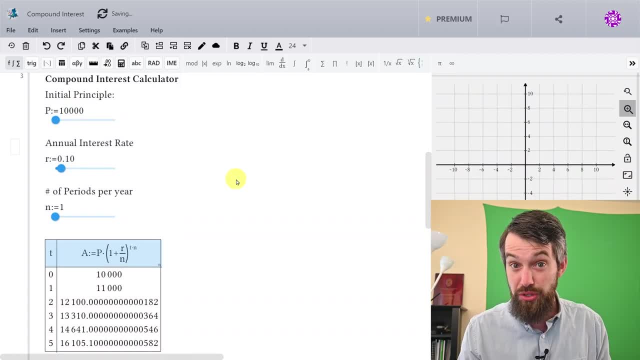 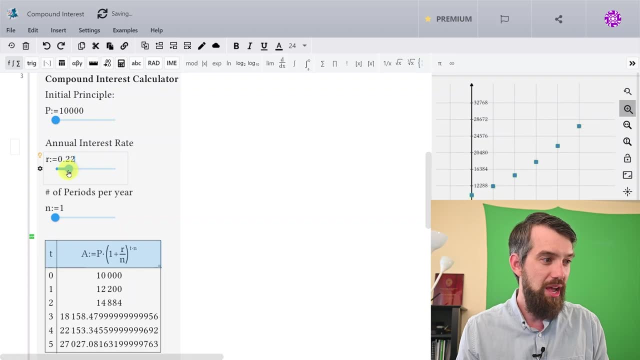 imagine- I hope this won't be the case, but imagine that you had $10,000 on a credit card, And credit cards typically have large interest rates. Let's slide the slider up to something. well, that's a little bit too much, But it's not uncommon to have, for example, 18,, 19,, 20%. 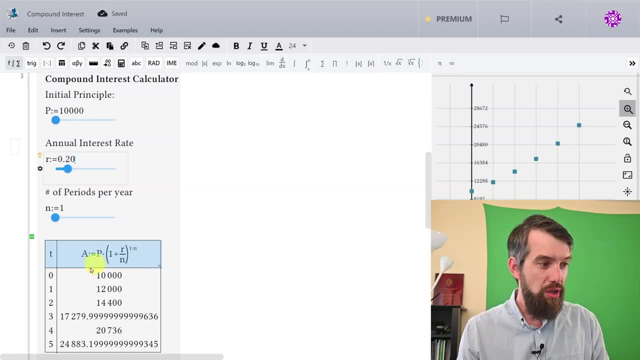 on a credit card. Well, if that's the case, your initial $10,000 that you would owe after five years is now almost $25,000.. Yes, this is ignoring that. for a normal credit card, you have to make a. 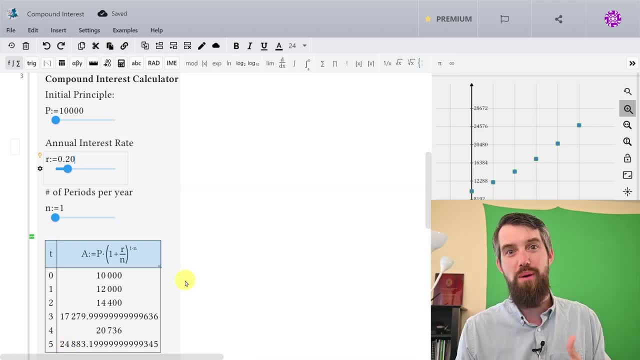 minimum payment every month. However, it shows just the power of compounded interest when it's working against you if you owe on a credit card where, when those interest rates start being high and you have compounding, then you start getting these really large numbers. This is all if it. 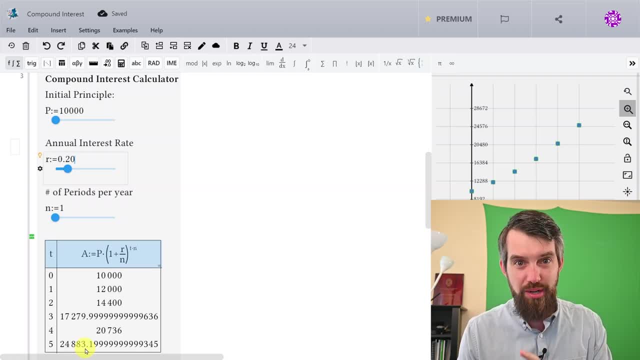 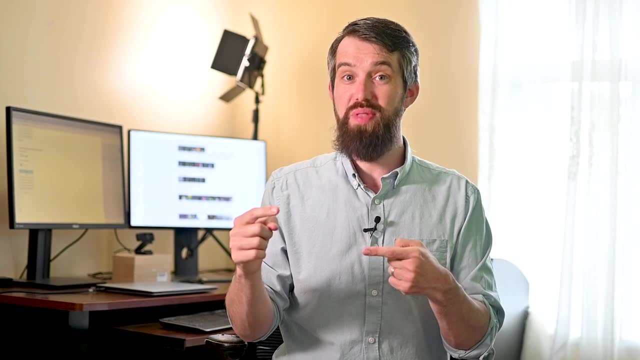 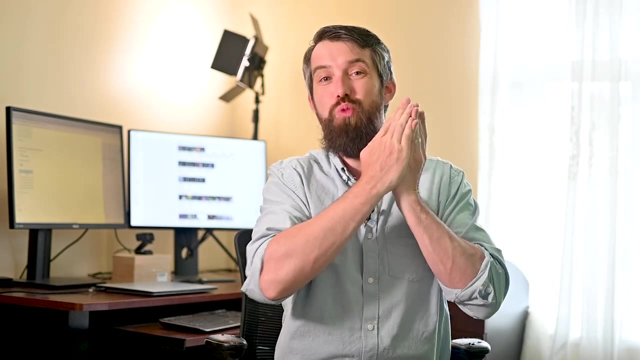 compounds once per year, But the story is going to get a little bit worse in a moment because we need to talk about what happens when you compound more often than once. One problem that occurs when you're trying to compare different types of compounded interest is that the value for the interest rate might seem wildly different, For example, if one person has a 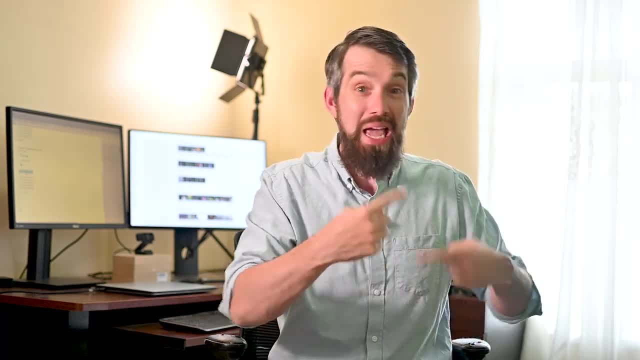 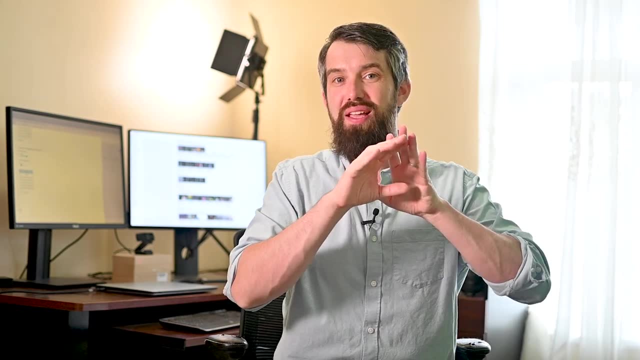 loan and they're compounding once a year, the interest rate might look way larger than the interest rate if you're compounding once a month, or once a week or once a day. So in order to try to compare everything on the same terms, we adopt a societal convention that all interest rates will. 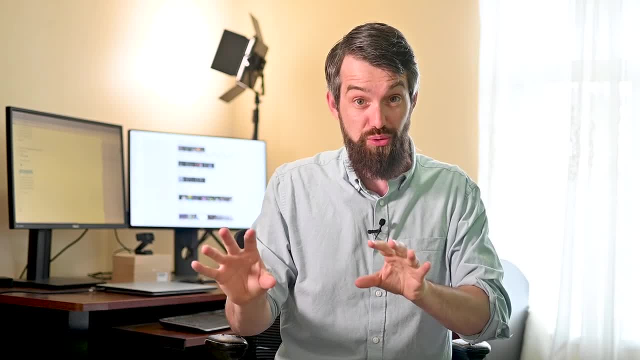 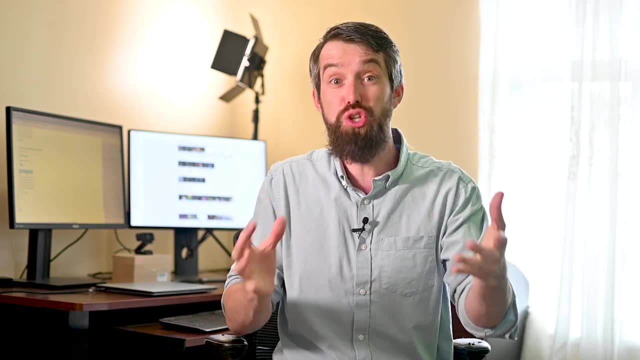 be spoken to for the most part. So let's start with compounding as annual interest rates, and then we're going to adapt the formulas when we want to deal with them compounding more frequently than a year. Let me show you what I mean. 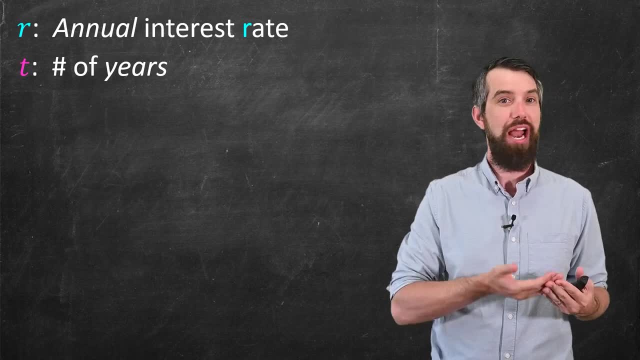 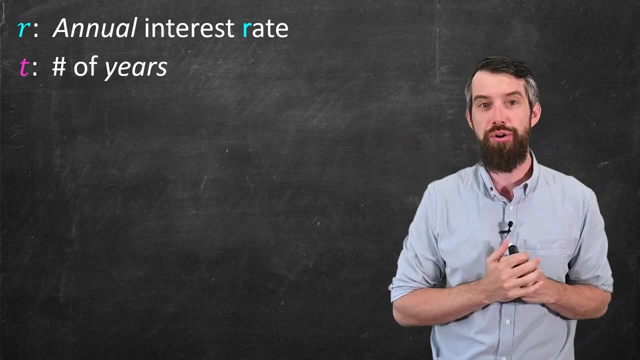 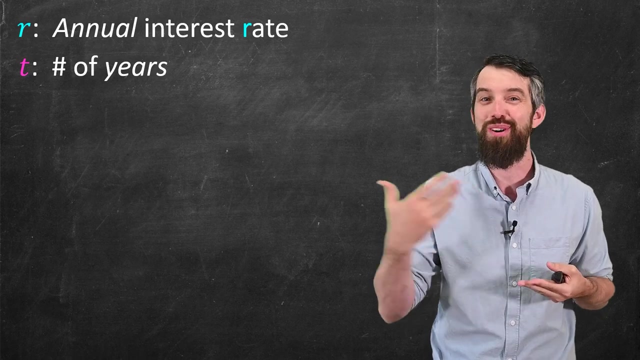 To deal with this, I want to again have the R and the T that we've seen previously, Except this time. I'm going to be explicit that the period is a year. here, R is the annual interest rate over a year and T is representing the number of years as opposed to a number of periods which might have. 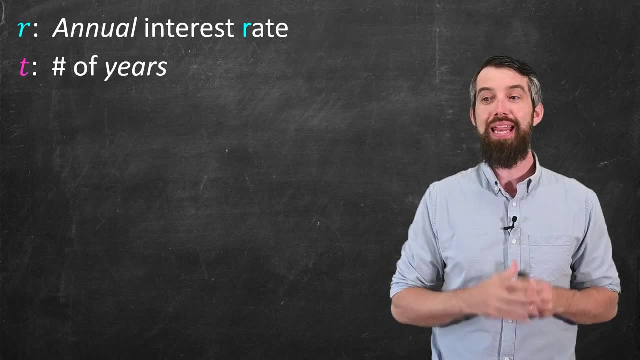 been less than a year. But then I'm going to go back to compounding and I'm going to go back to compounding and I'm going to have to add a new thing. I'm going to let N refer to the number of periods in a year. So, for example, 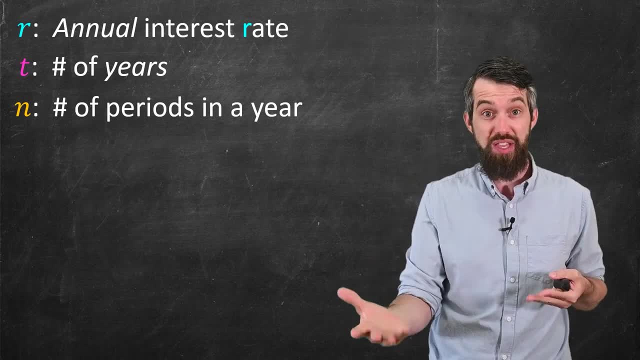 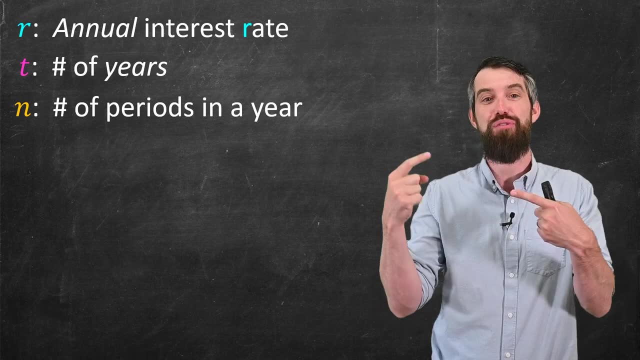 if you're compounding monthly- there's 12 months in the year- your N would be 12.. So you sort of have this annual interest rate, but then you're going to be compounding it every month, so you need this value of N equal to 12.. Now the old formula, so I haven't made adjustments to it yet. 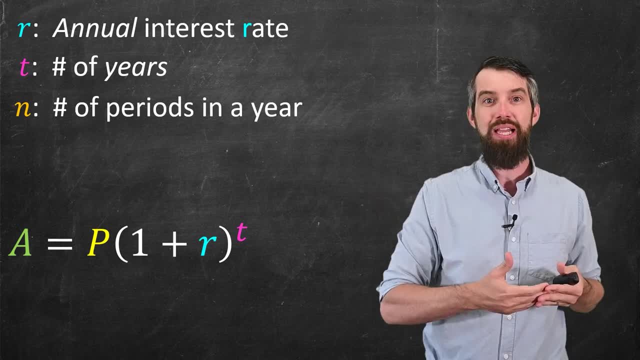 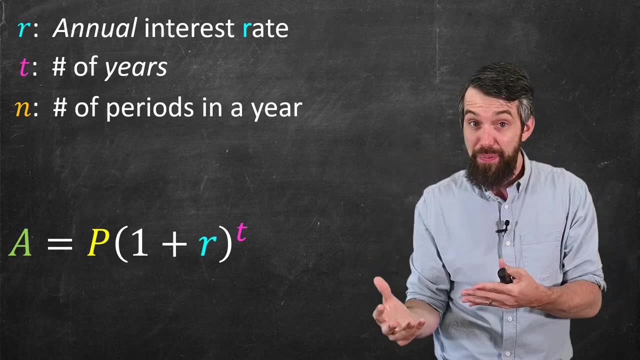 the old compounded interest formula was this: P times one plus R to the power of T And basically this formula is the N equal to one case. But I need to see how to adapt this if you have multiple periods in a given year, And what I'm going to do is I'm going to tweak it in. 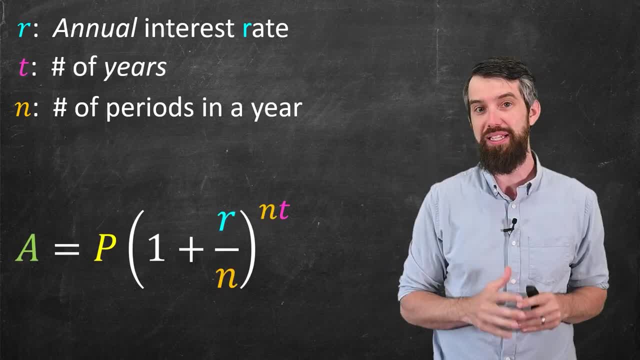 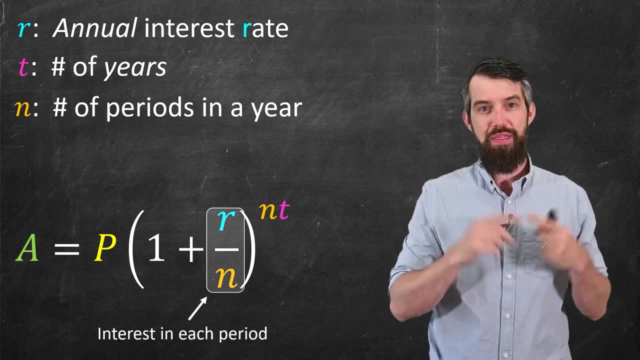 two places. I'm going to divide out by an N and I'm going to multiply an N in two different places. What's going on? Well, the first is I have, instead of R, I have R divided by N. The idea here is: 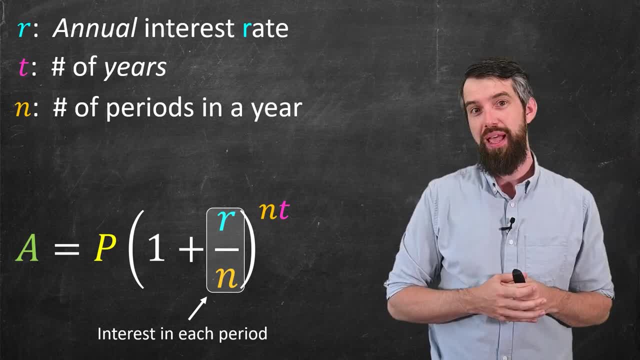 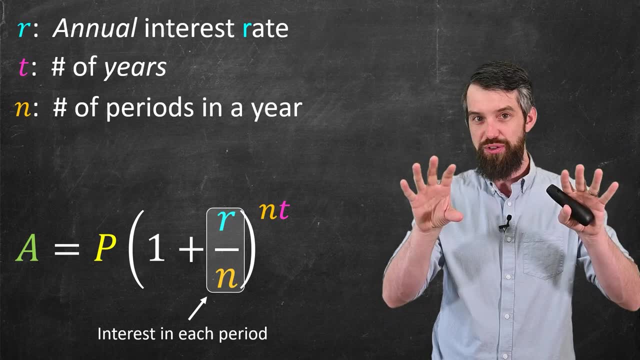 suppose you have an annual interest rate R of 10%, And what we're doing is, if we compound, say monthly, where N is equal to 12,, you're taking that 10% annual interest rate, you're dividing it by 12, and that's how much. 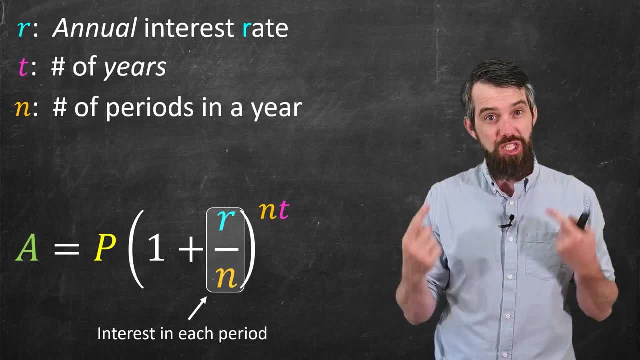 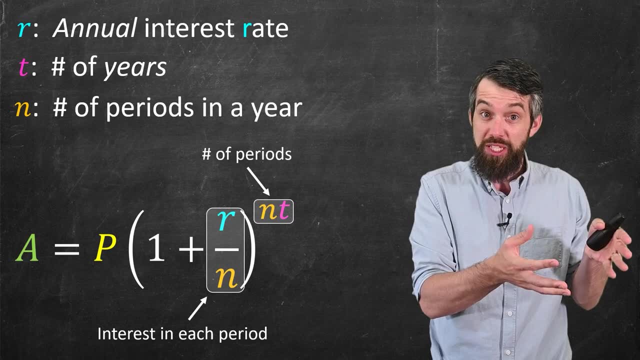 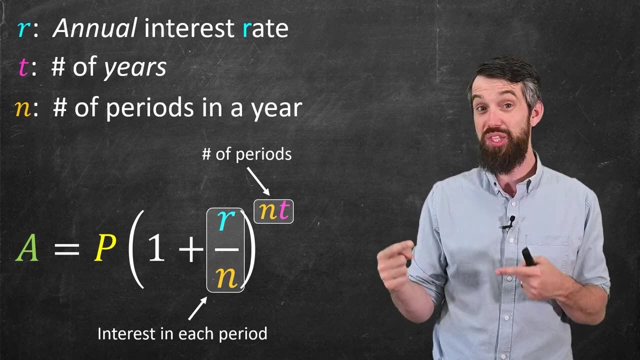 interest you're applying on each month And then in the exponent where we've got the N times the T. this tells you the total number of periods. N is the periods per year, T is the number of years. so N times T is the total number of periods And the idea is- I need to take this compounding. 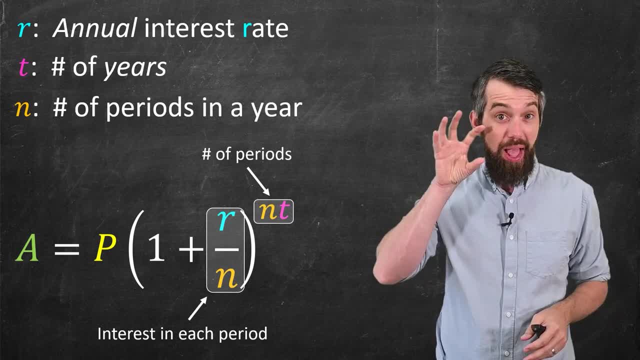 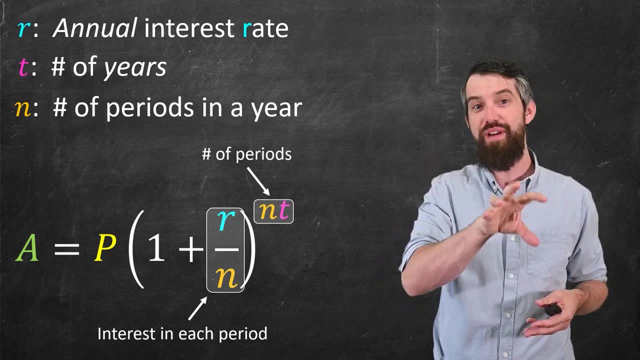 factor that one plus R divided by N, and I need to multiply it every single period. For example, if there's N times T periods, you want it to be one plus R divided by N to the power of the N times T, So we've modified our previous formula. This then leads to the 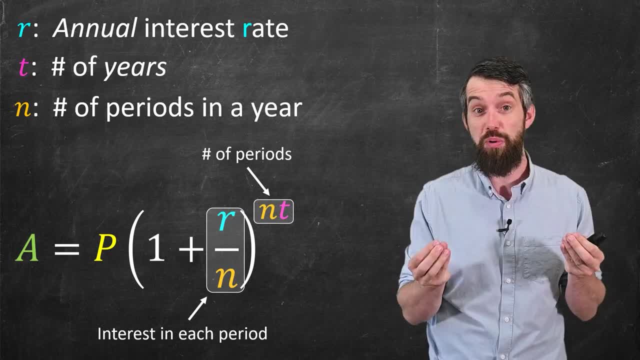 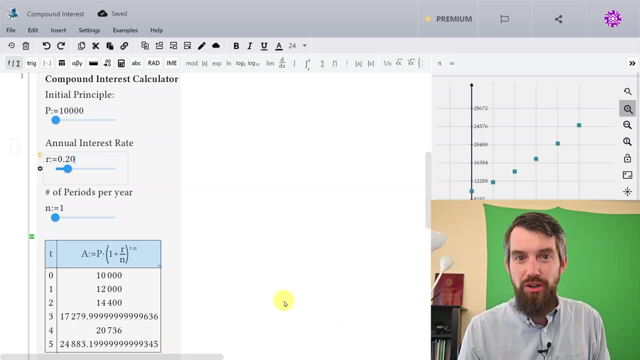 following question: What N should you choose? What N gives you, for example, the most amount of interest? Let's go back to our MapleLearn workbook here and I want to increase our crazy credit card example, where we started with $10,000 and it was 20% per year. But now I'm going to take 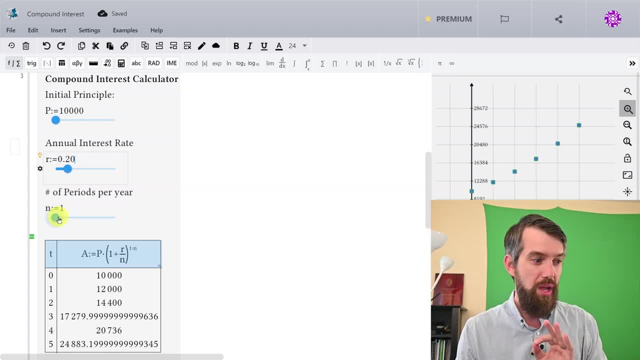 the N equal to 1, the number of periods, and I'm going to increase it. Notice that right now, before I increase it, that after 5 years you'd owe $24,883.. If, instead of 1, I write 12 here: 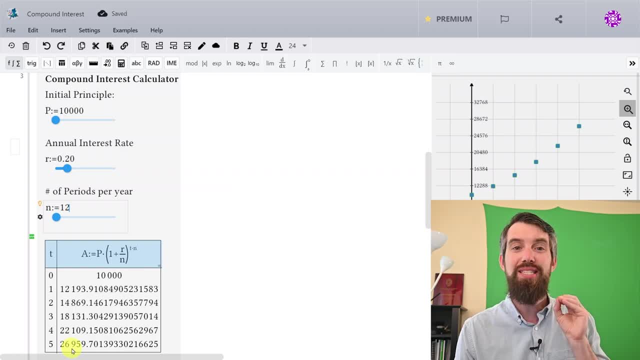 now it's increased and after 5 years you owe almost $27,000.. And this shows that when you compound more frequently, the amount of money that you owe goes up at the same interest rate and same initial principle. Well, how bad could this be? 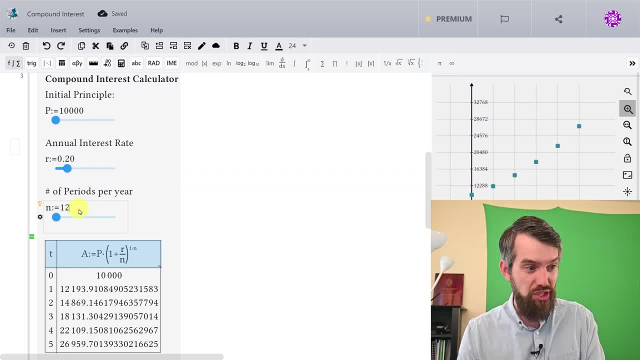 For example, what if, instead of monthly, you did it daily? So instead of 12, you go 365 here, And actually this has increased. It's a little more than 27,000, not a little less than 27,. 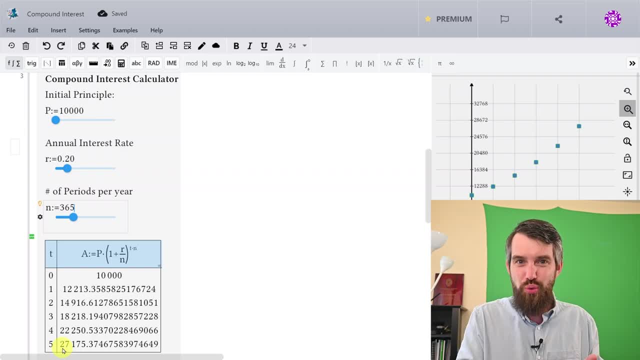 but not actually as crazy of an increase from 1 to 12.. And in fact, if you wanted to go kind of extreme and say I don't know how about 10,000 divisions per year, it actually barely changes the final value after 5 years. If you want to go kind of extreme and say I don't know how about 10,000 divisions per year, it actually barely changes the final value after 5 years. 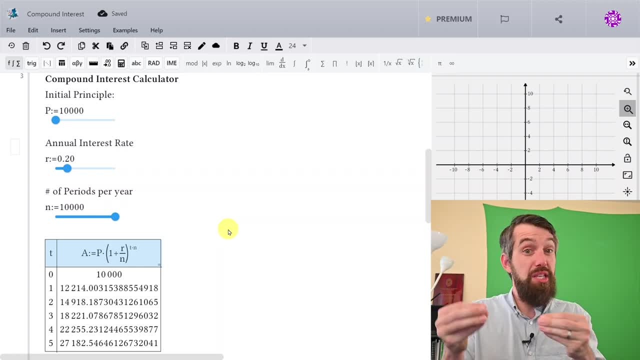 And the idea here is that as you increase the number of periods per year, the amount goes up, but it starts to slow down in how it goes up. So then this sort of begs the question: well, what happens if I increase my frequency of compounding as much as possible?